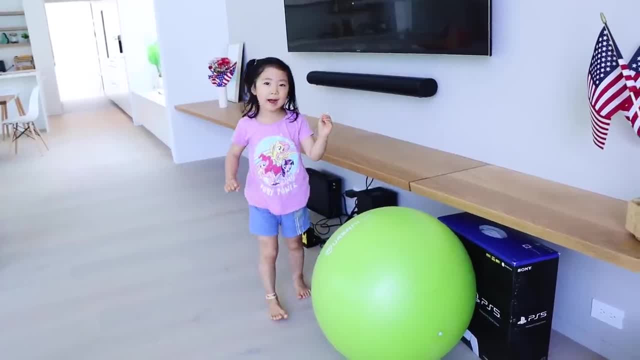 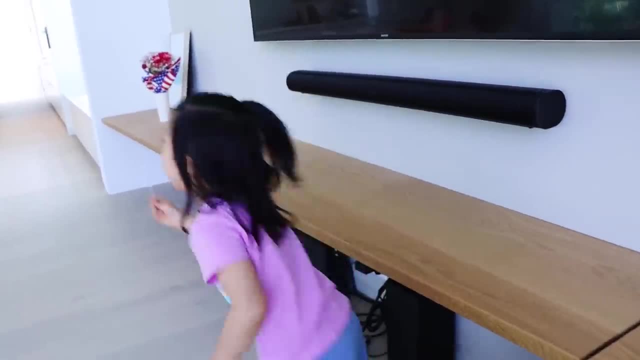 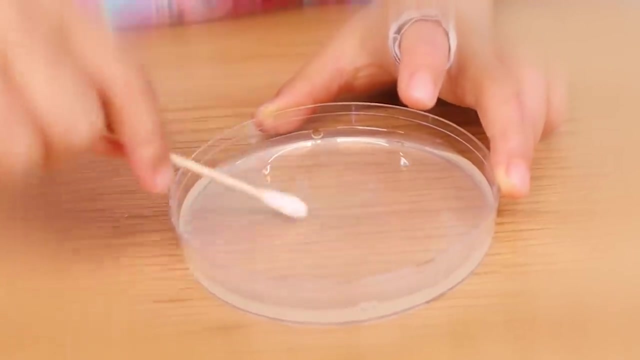 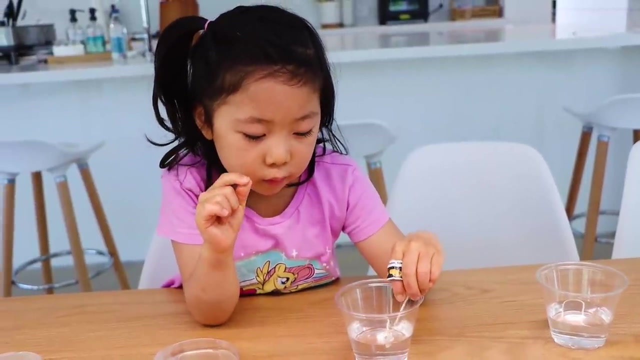 How about germs? This ball came with a house. Let's test it by cereal. Put it inside. Let's put the cereal on the plate. B-A-L-L. Germs, germs and Sarcoses. Germs, germs and Sarcoses germs. 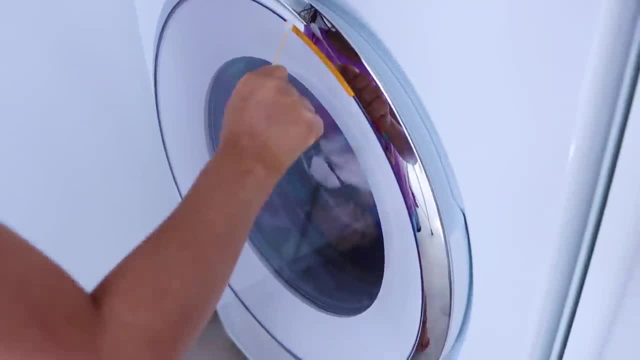 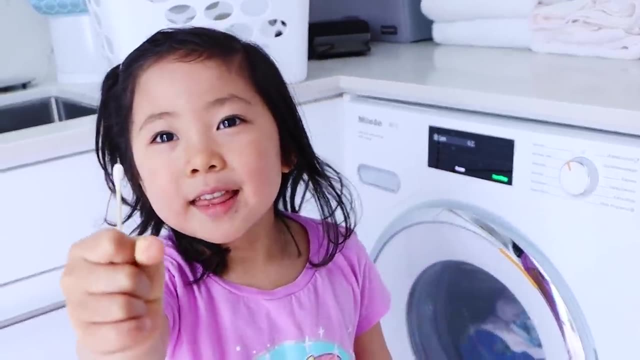 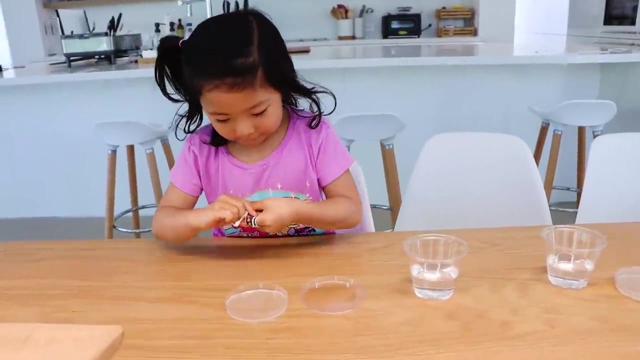 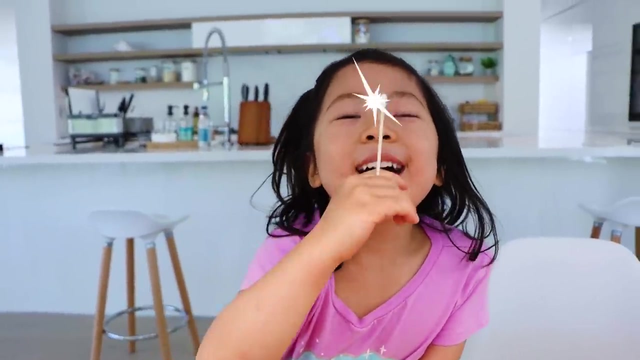 And water makes germs, Germs, germs and Sarcoses, germs, Dirty water. Now let's go put. this is to see if there's dirt, Now put it on the plate. Okay, done, Washing machine. 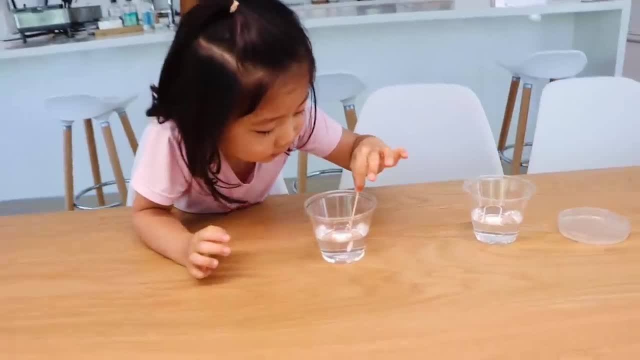 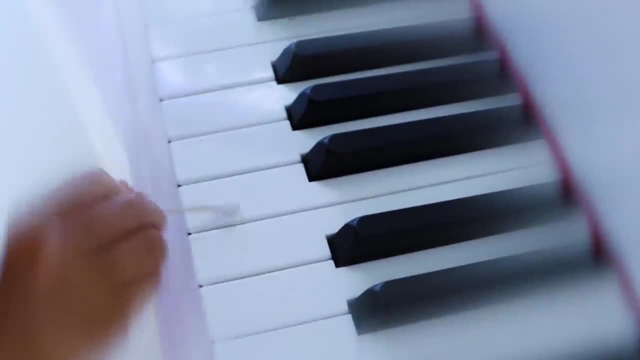 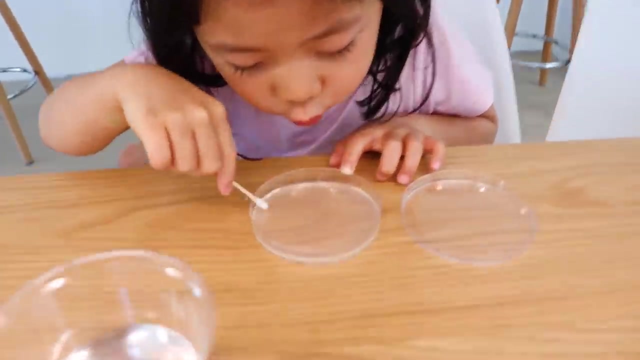 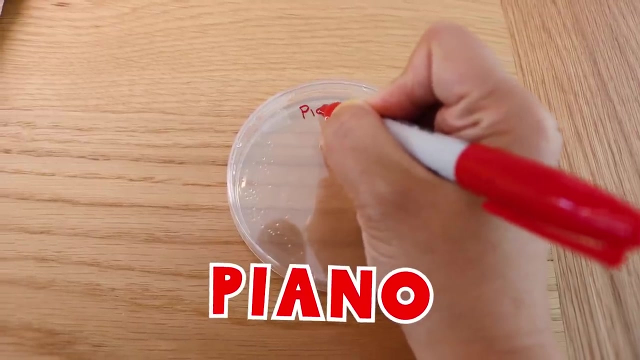 Okay, ready, my turn. Dip it in water. Let's test the keyboard if it has germs. Now I'm putting it in the plate. Look at all the germs. Piano P-I-A-N-O piano- My turn again. 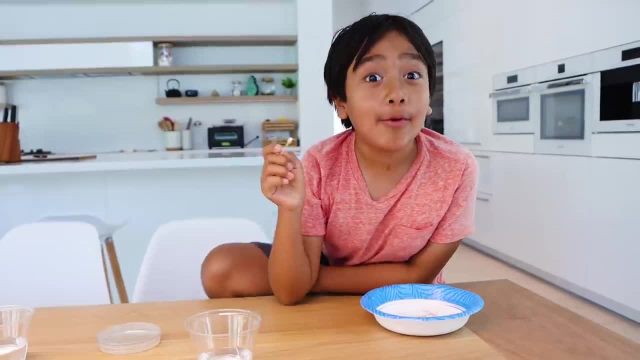 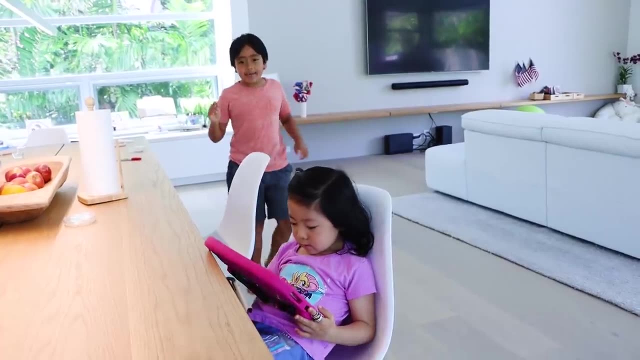 Put it in the water. I think I know who I'm going to test. I'm going to test Kate's iPad because she hasn't cleaned it in a long time. Okay, let's go. Okay, Kate, I'm going to test your iPad for bacteria. 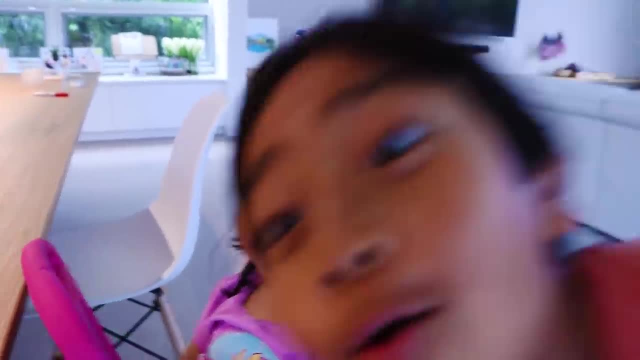 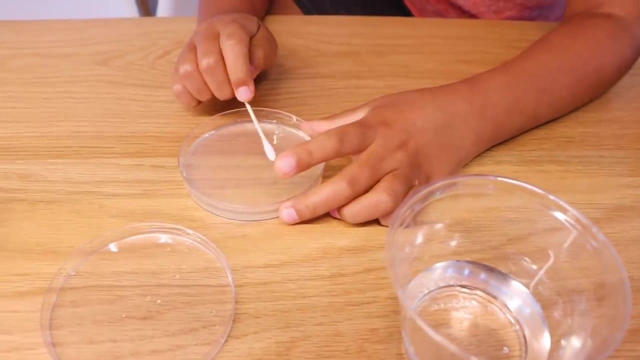 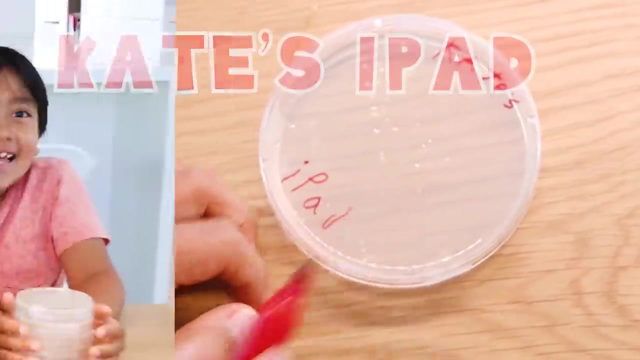 I hope there's no bacteria on my iPad. I know why Bacteria on Kate's iPad, Okay, Okay, Okay, I'm going to put this on Kate's iPad. Now we're going to put this Adder plate into the box. 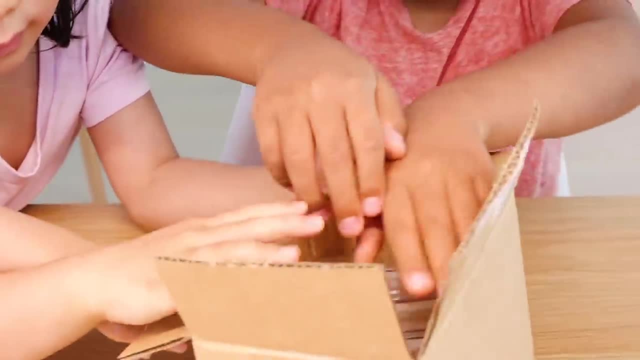 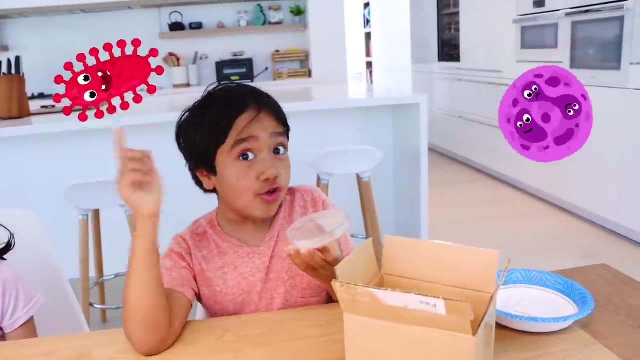 The box, The box, Oh oh oh. I almost forgot. We have to keep a plate for control. Let me go Basically. this one has no bacteria inside. Now let's tape the box. Okay, Kate, you tape it first. 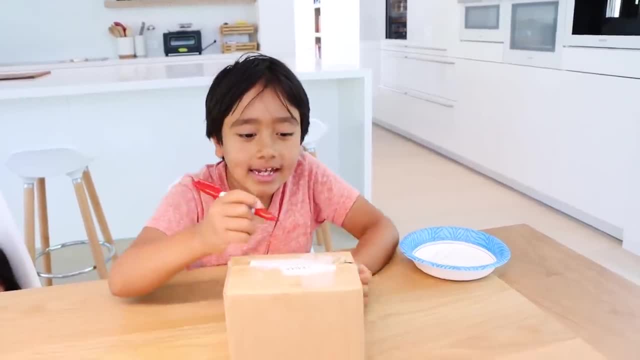 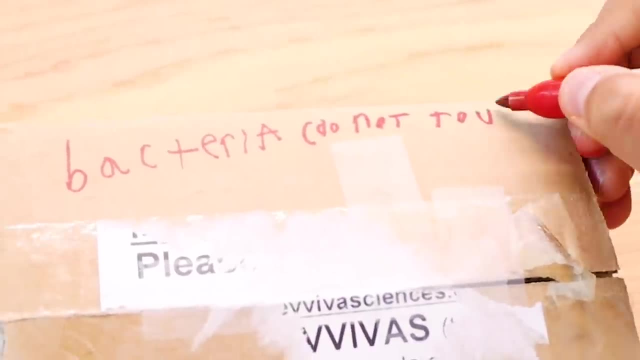 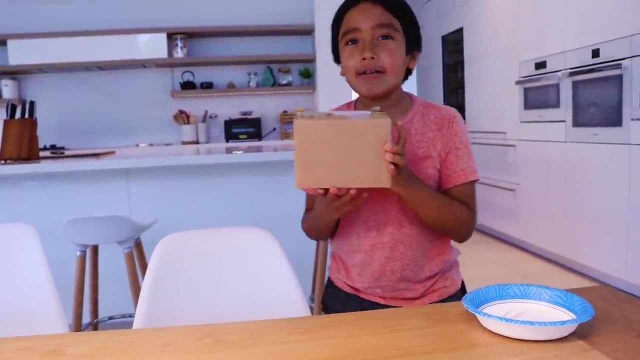 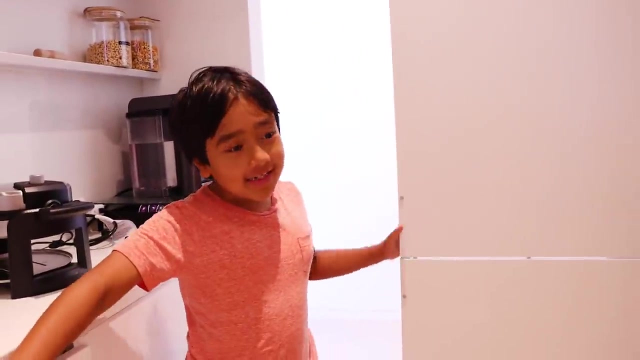 And there And there. Now it's labeling time. Bacteria do not touch. Now we're going to put it somewhere safe. Okay, Hmm, where is somewhere safe? See you in seven days, bacteria, But don't open it and try this at home. 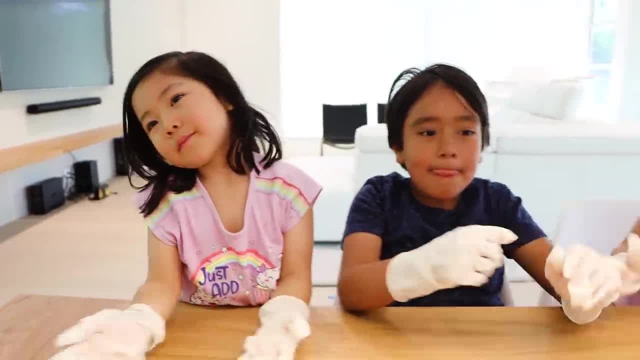 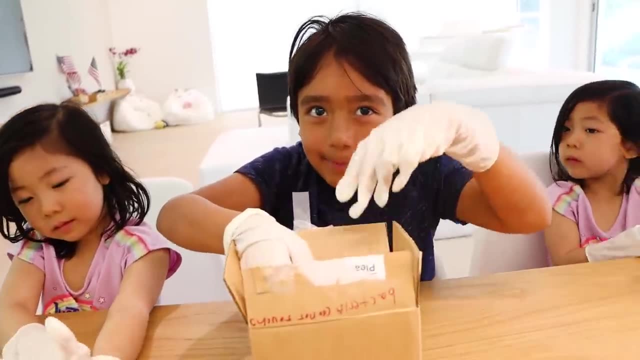 You have to eat close. You have to eat gloves to try this at home, That's right. Yeah, protect yourself with gloves. Okay, guys, it's been one week Now we're going to take the bacteria out and see if there's any bacteria. 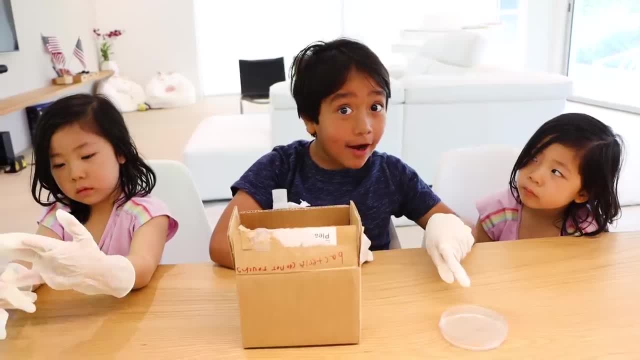 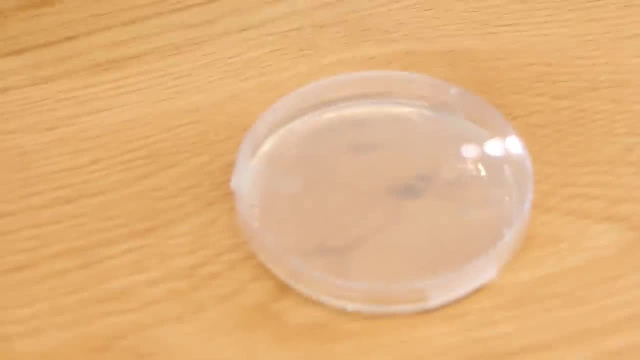 Hmm, Okay, This one has no bacteria on it because it's the control, So we didn't swab it for any bacteria. Oh, so these are good, because that means this: these dish are good to go because there's no bacteria grow, because we didn't swap it. 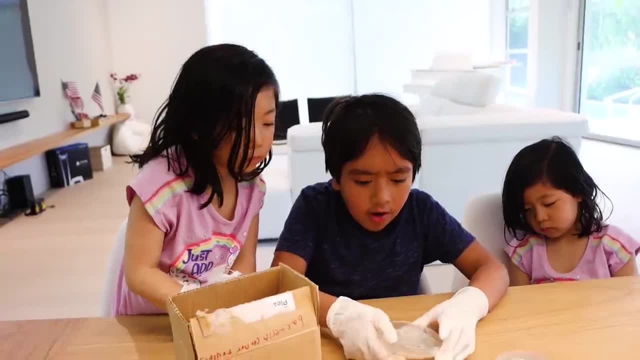 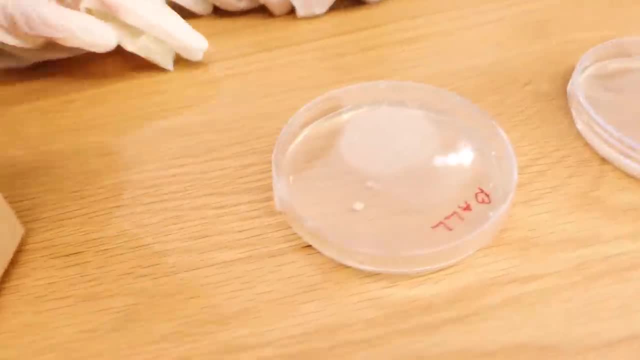 Okay, Okay, Okay, Okay, Okay, Okay, It's a ball. Whoa, that's a lot of bacteria. Wait mine, I got it. Yeah, so this is the one Kate did. Look at the ball, guys. 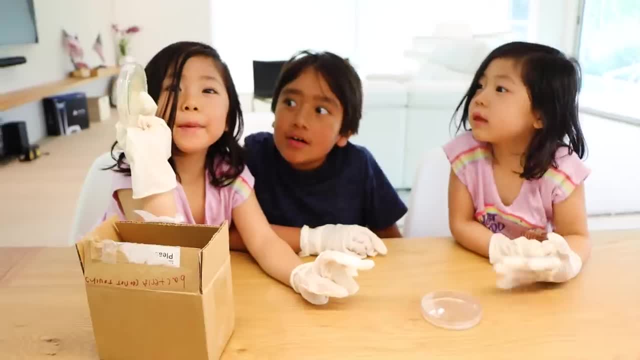 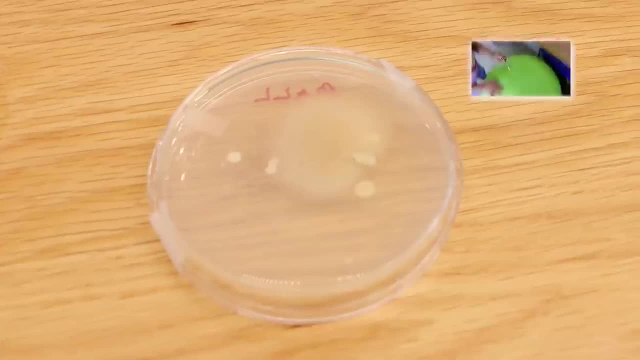 You guys see that bacteria right there. Yeah, Yeah, Ew. That's a lot. So much bacteria. Ew Right, Ew gross, Ew, Ew Gross. Even the ball that actually came with the house had bacteria in it. 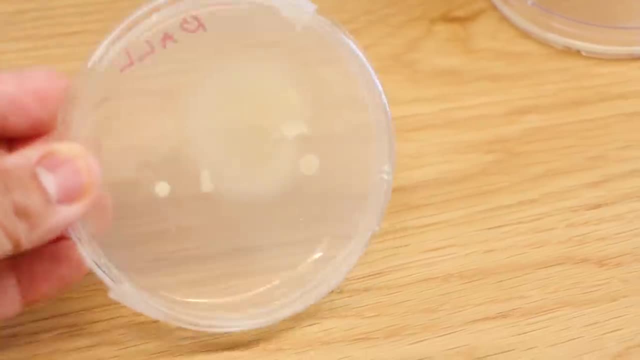 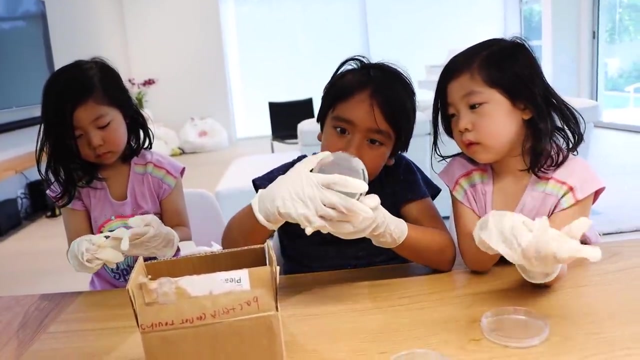 So after we finish playing, we probably need to clean the ball. You guys see those bacteria on there. Yeah, Okay, Oh, this one doesn't have that much. Which one is that one? It is the wall, Oh, the wall that Ryan swabbed. 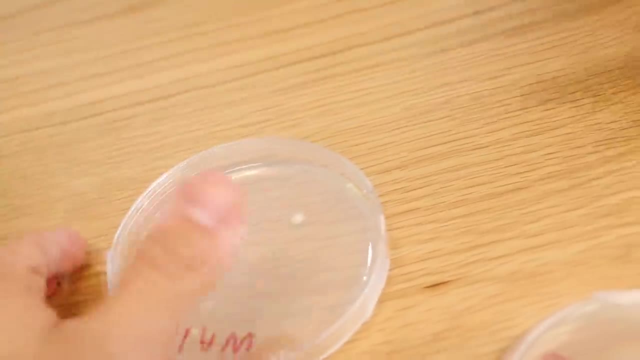 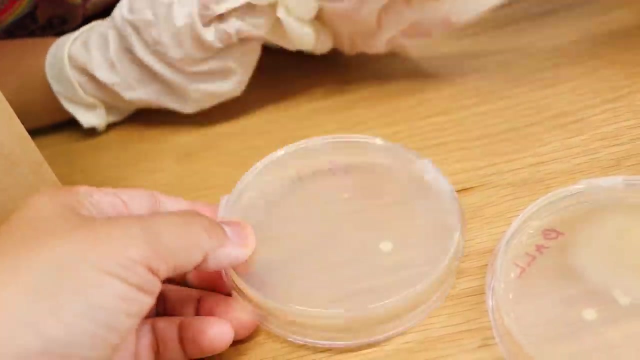 Okay, Oh, Oh yeah, look guys. So there is a little bit colony there, Yeah, But not a lot of growth. Yes, Maybe if we wait longer it will grow. Wait less than this one, at least. Oh yeah. So there it is the wall. 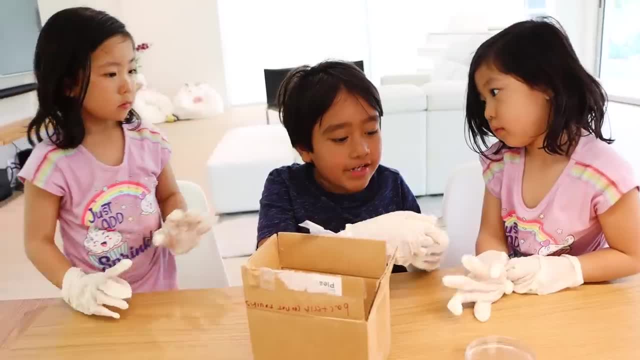 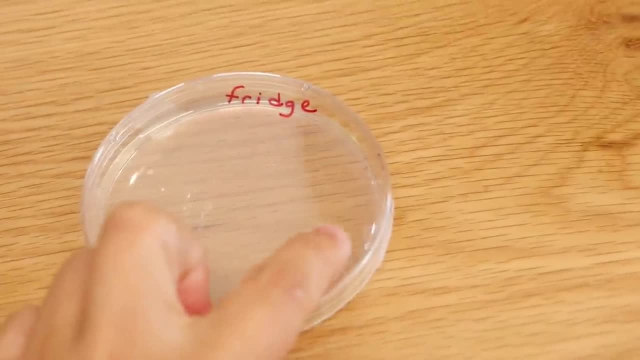 Okay, Which one is that one? The fridge doesn't have that much on it Really. Yeah, That's nice, There's like one. Yeah, Oh, that's bad luck. Just that one colony right there, only, So okay. 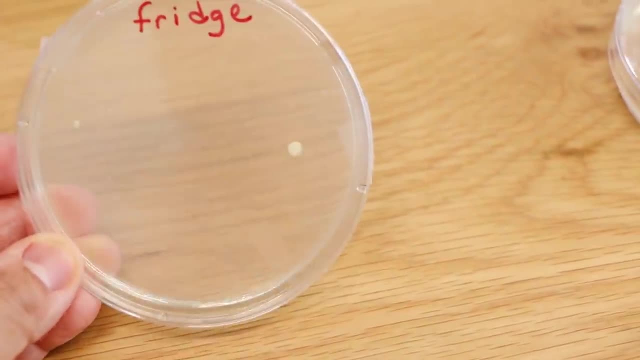 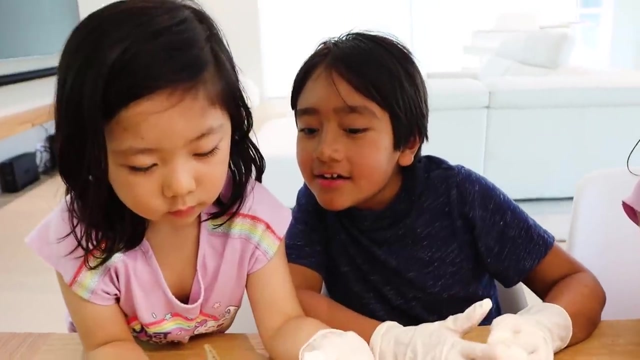 But it's still a little dirty. So I mean we probably need to clean the fridge, right? Yeah, There's bacteria everywhere. Yeah, See what this one is. It is Kate's iPad, Oh, Kate's iPad, Ooh. 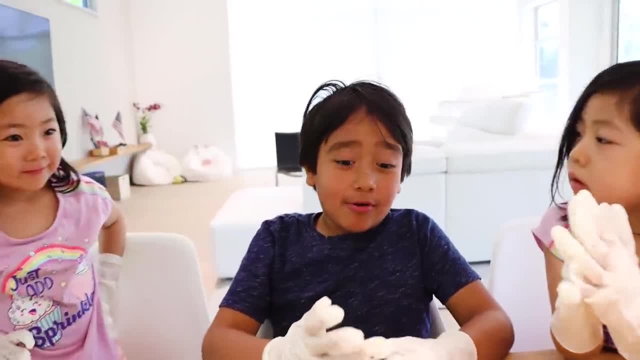 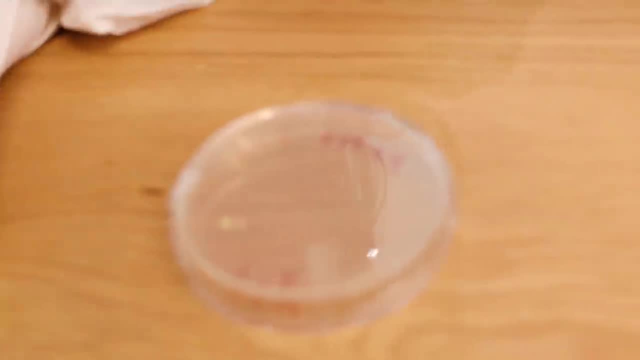 Oh, it actually doesn't have that much. Yeah, Kate's iPad is more greasy than bacteria. Super, super greasy, Yeah, But is that dirty? Not that much. Let's see here, Right? But still, Kate, look, there's still bacteria on your iPad. 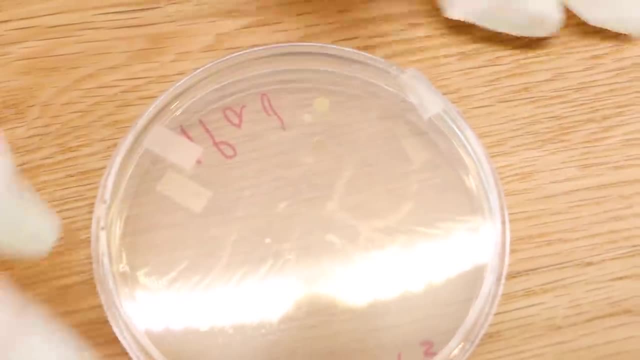 Do you guys see, right there, There's a colony spot right there. It's almost like I cleaned it not too long ago. Oh, you did. Yeah, You have Kate cleaning. That means we got to probably clean everything we touch right. 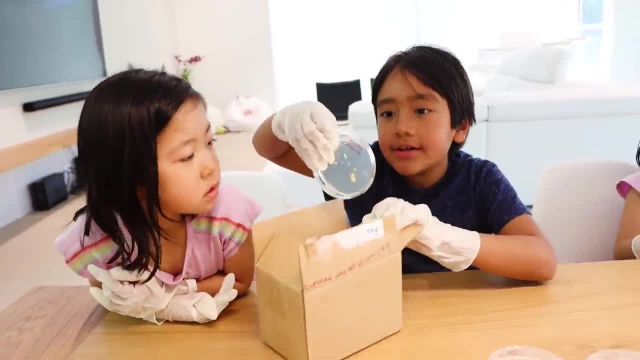 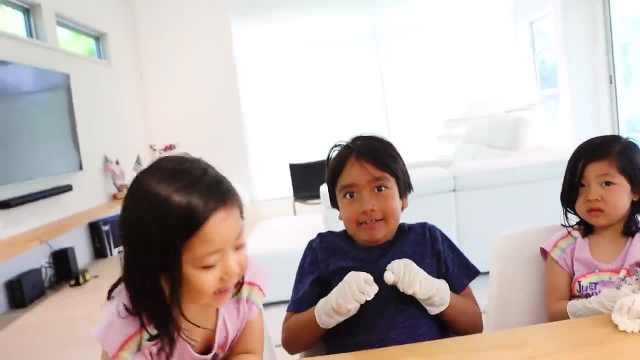 Yeah, Yeah, Okay, let's see what this one is. Oh, that one looks like a lot. It's the washing machine. Oh guys, Yeah, That makes sense, because what do we put in the washing machine? Oh, Clothes. 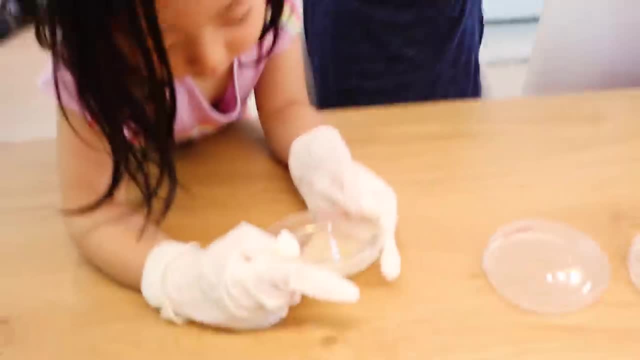 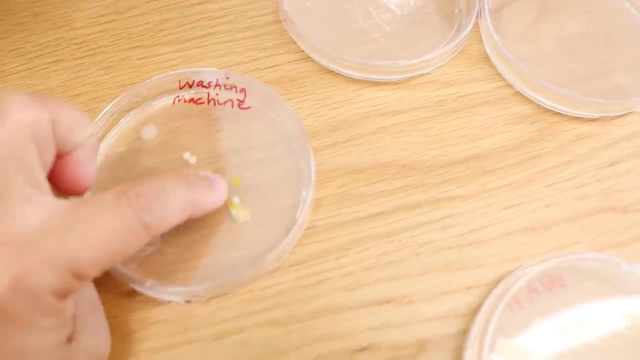 Dirty clothes? Yeah, We put in clothes, That's right, So that's why I can see the germs. There's some germs, Yeah, See, this is interesting because, look, this is like different color of bacteria. 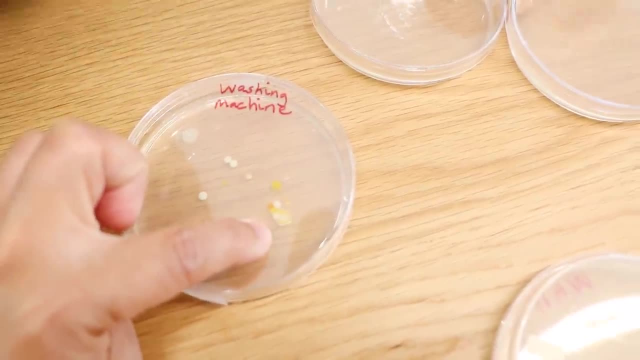 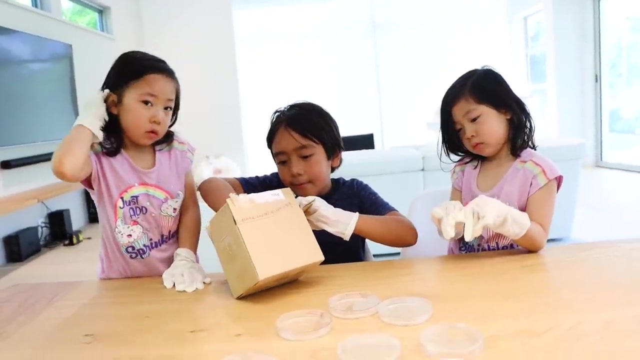 So different type of bacteria. There's a white colony and there is a orange colony and a yellow colony too. Do you guys see it, the difference? Okay, one more. Look, there's a black color in it- Black. 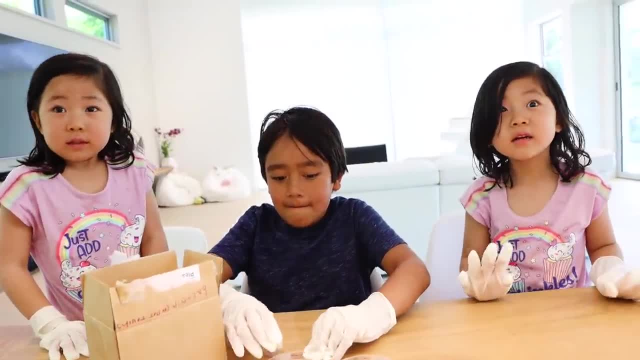 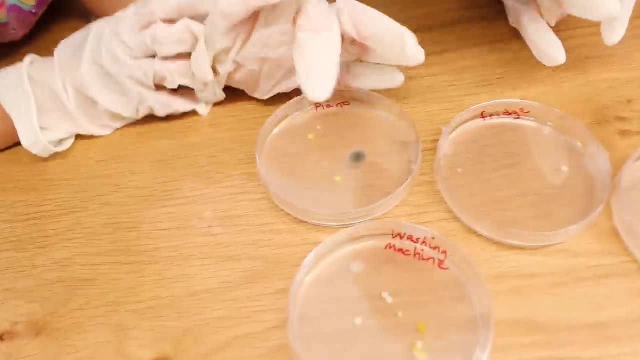 It's like piano. Oh, Piano, Piano is dirty. Oh, Emma, we got to clean the piano. There's a big one like super black one. There's a black one. Oh, there's a different type of bacteria colony. 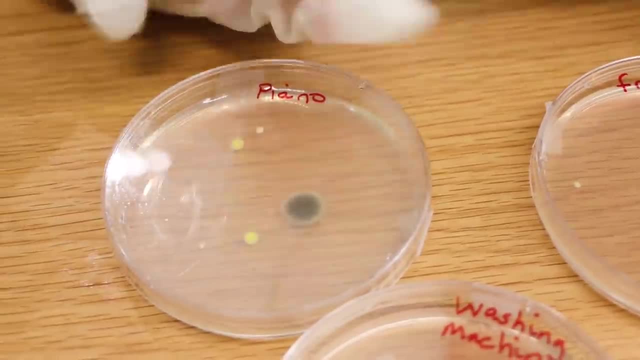 It's like a black color. Do you guys see it? That's big. Why does black germs do that? I don't know. It's just different type of bacteria, That's why. Okay, So what did we learn, guys? 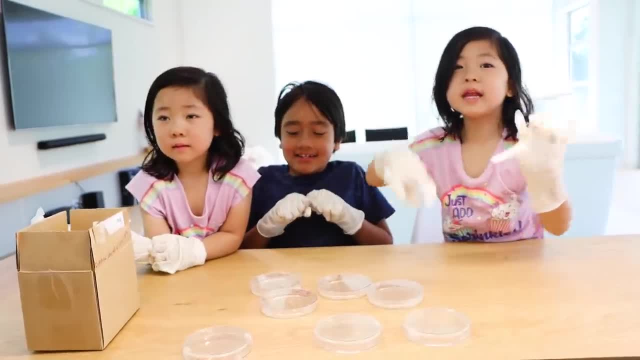 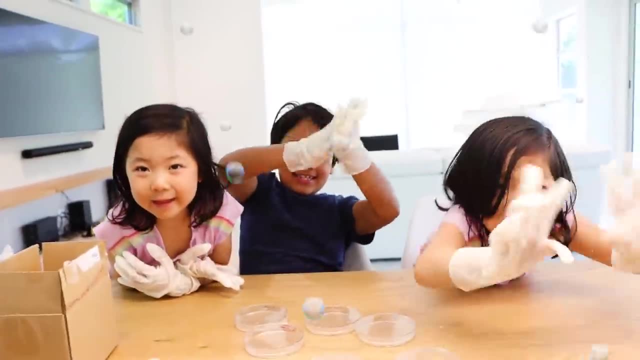 Wash things that is dirty. Yeah, That's right, Wash things that you touch. And then also, besides washing things, you should also wash your, Your Hands, Your hands, Your hands, All right Hands. Thank you for watching. 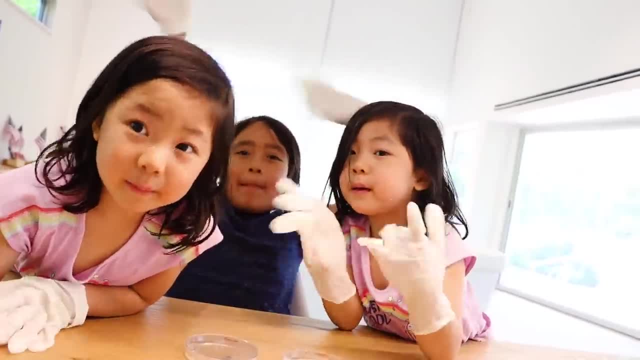 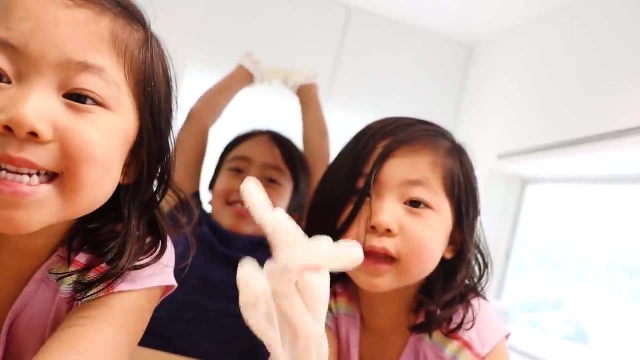 Thank you for watching. Remember always stay happy and bright. Bye, Bye, Bye, Bye, Bye. Thanks for watching. I'm going to keep videos down below. I'm going to keep videos in the screen. Bye, Bye, Bye.